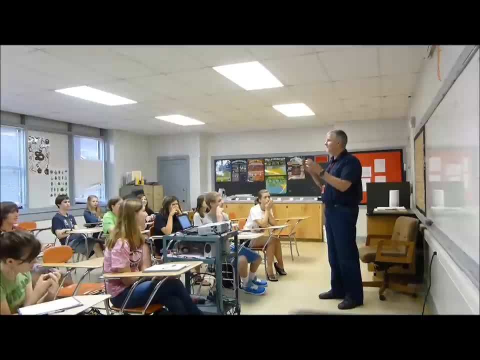 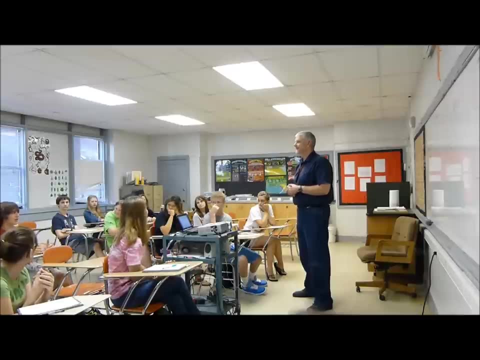 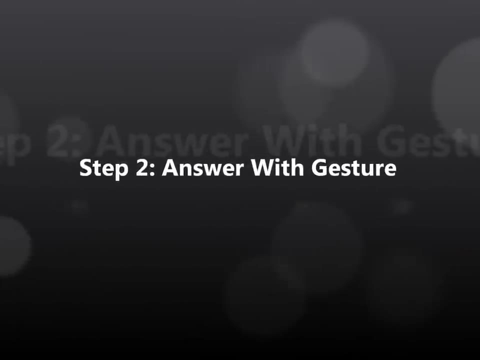 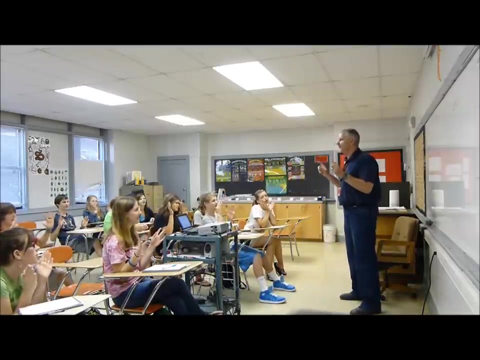 A chemical is anything with a defined molecular composition. What did I say? A chemical is anything with a defined molecular composition. That's good. Keep it deeper. Now, mirror, Say it with him: A chemical, A chemical Is anything. 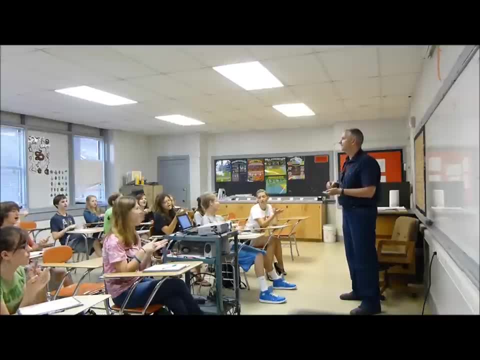 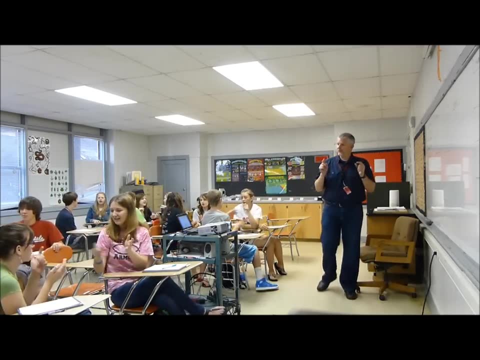 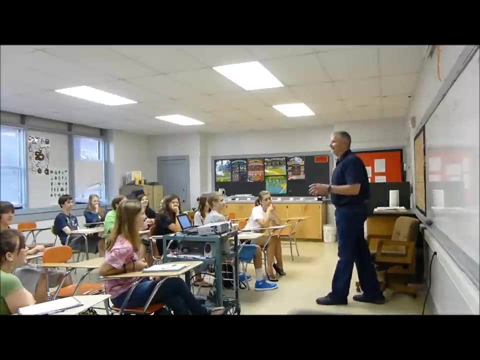 Is anything With a defined molecular composition. With a defined molecular composition, Teach that in your part. Ready Go, Teach. Okay, So we're talking about the molecules inside the chemical. So the defined molecular composition means we're going to be able to tell you. 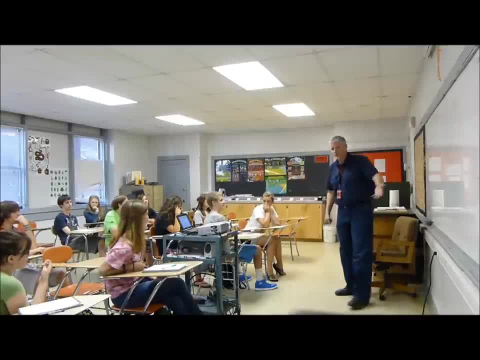 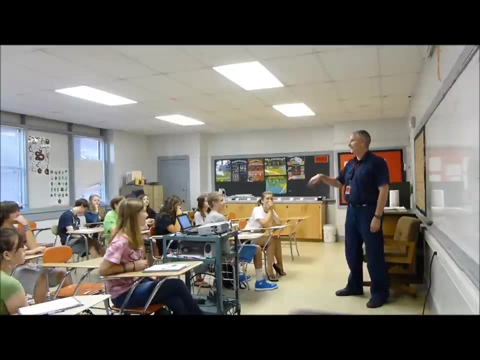 exactly what, What it's shaped like. What it's shaped like What its composition is right, That was pretty good. Give him a five-fingered uh-huh, Uh-huh, So. defined molecular composition. Defined molecular composition. 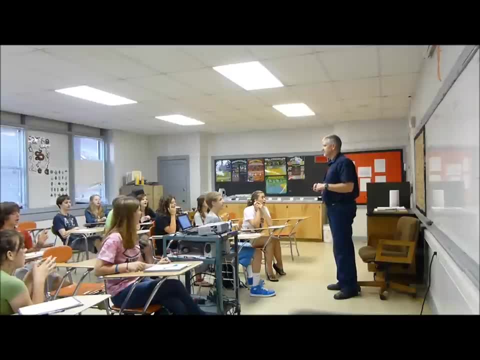 Means. I know what elements are in the chemical Means. I know what elements are in the chemical. One more time: Defined molecular composition. Defined molecular composition Means. I know what elements are in the chemical Means. I know what elements are in the chemical. 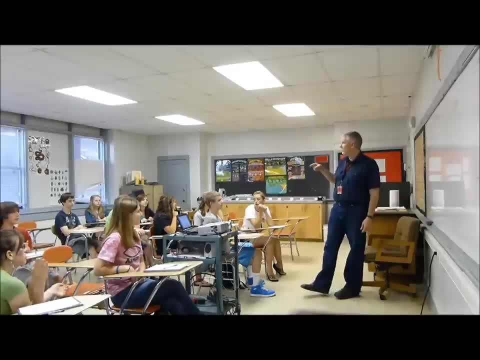 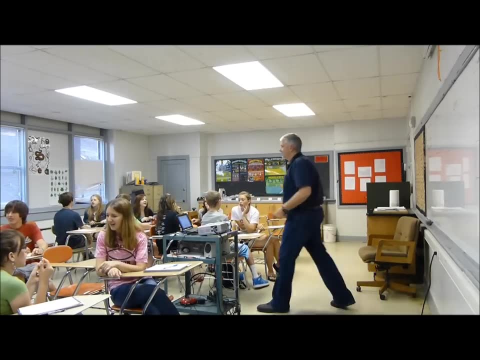 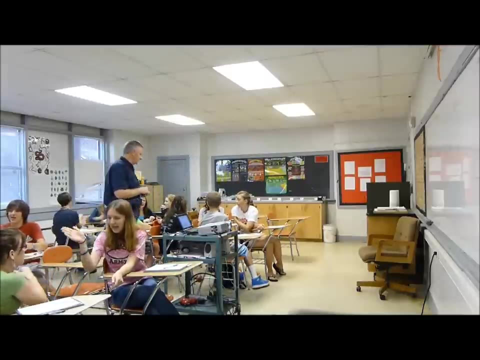 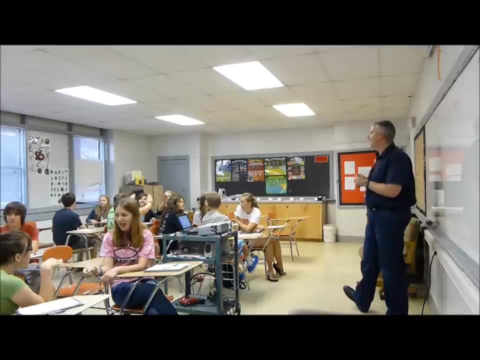 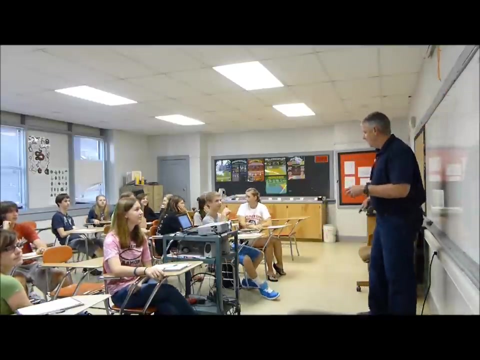 Let's do that. one Teach okay with a switch Tag team. That way you can make sure that each of you knows it Ready Teach Class. Yes, I'm seeing some good work here on the tag team. I'm going to have to give you credit for that. That's better than I even thought you'd do, And I expect a lot of you. 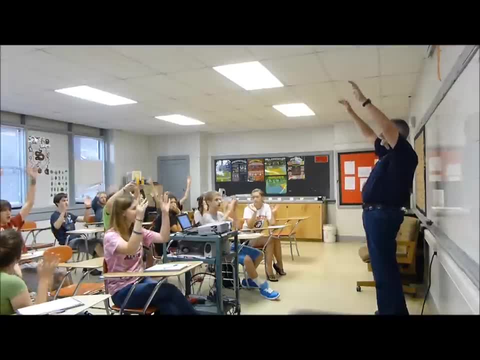 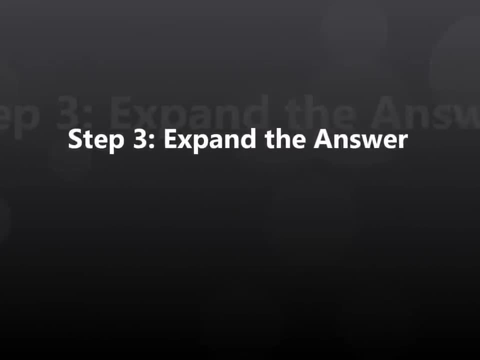 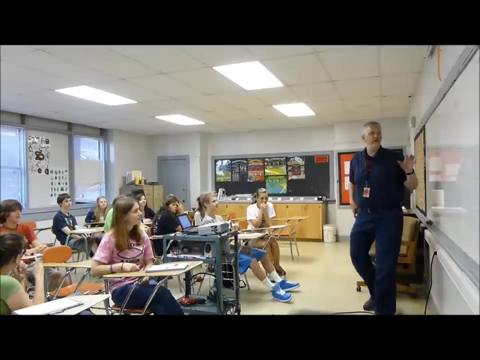 Give me a one second party fireworks Ready. Sizzle, Sizzle, Sizzle, Class, class, class, Yes, yes, yes, Alright. so when we talk about a defined molecular composition, we're going to know exactly what's in the chemical. So if we look up here at this, here's a couple of examples, Sammy. 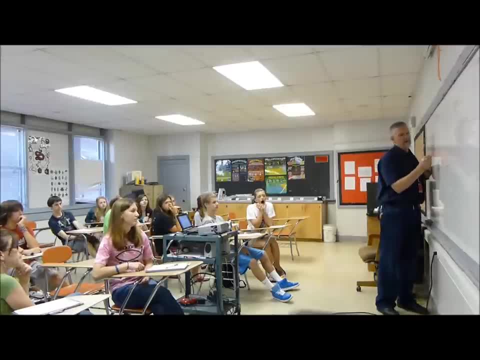 Water, Water. First one is water, So it's going to be. how do we define this molecular composition here, Heidi? what's the one with that Water? This is going to be water. How many of these do we have? 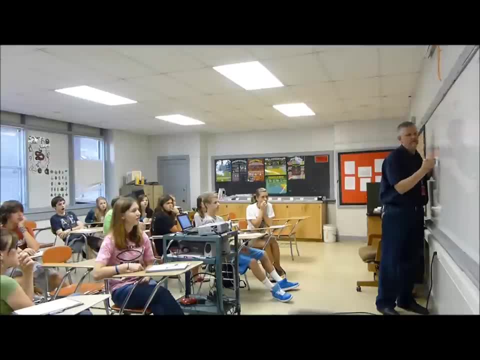 Two hydrogens. Two hydrogens, So that's H2.. One oxygen: One oxygen, That's O. Now, if I'm a chemist and I look at this, can I tell exactly how much of each element is in this chemical? 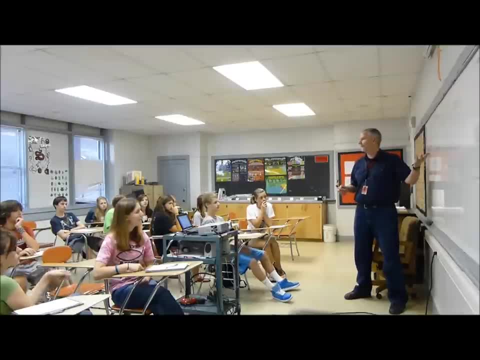 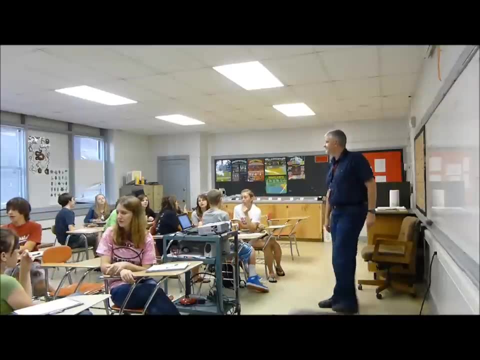 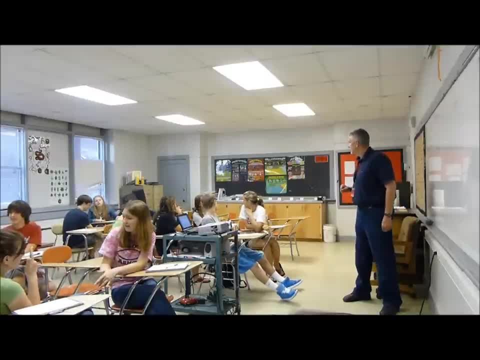 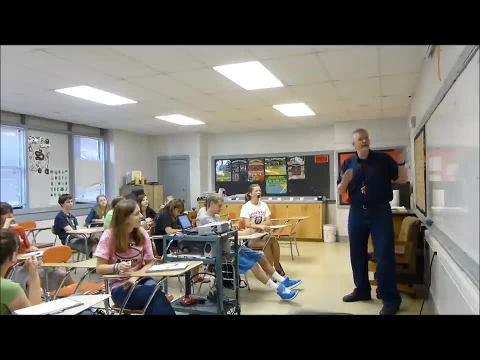 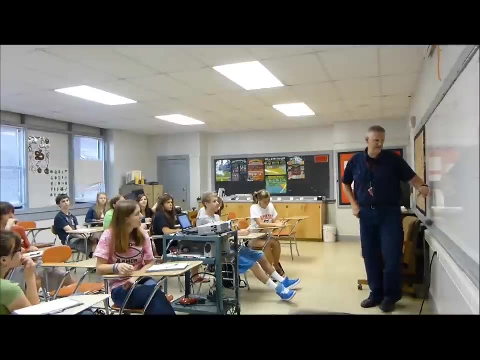 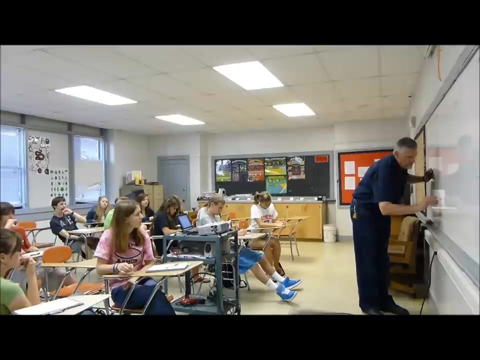 Curry: Yes, Yes, Nicely done. So we got the first one, and now let's look up here again. Now, what's this one down here? Let's go with, right here: Carbon dioxide, Carbon dioxide. Very good, So we can write down the word and what's the chemical formula here. 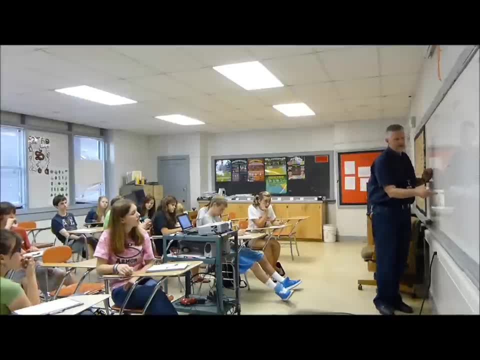 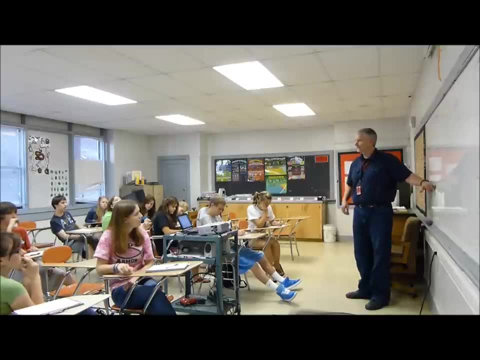 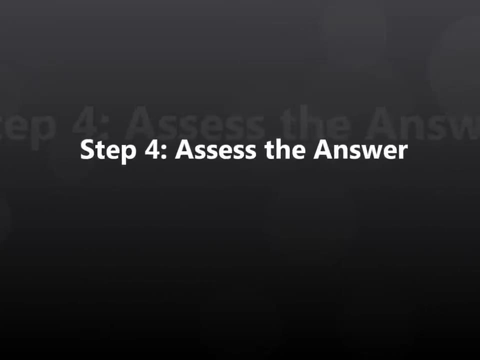 CO2. CO2, one carbon, two oxygen. Does this define what's exactly in this compound? Yes, And so does this make this a chemical. You mean, give me a thumbs up if it's a chemical, a thumbs down if it's not. 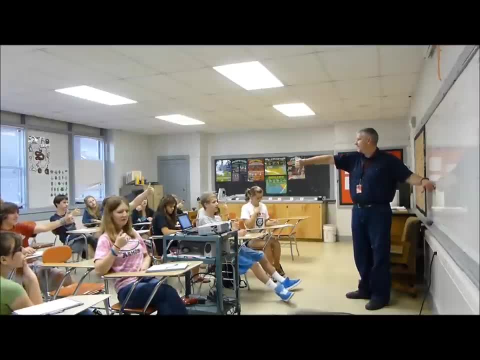 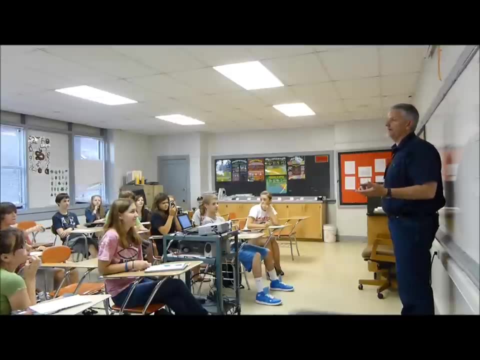 Is it chemical? Yeah, Yeah, whey, no, whey, Whey, Whey, no, whey, Whey, Whey, Whey, Whey. You guys are right on the money. What about carbon dioxide? Is carbon dioxide actually a chemical? 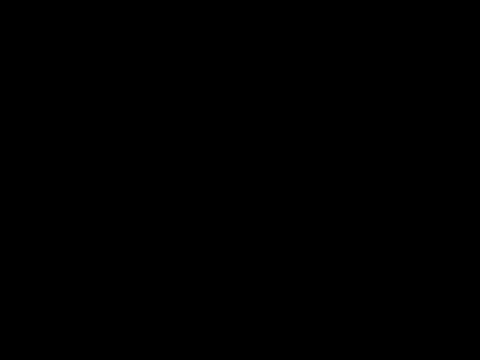 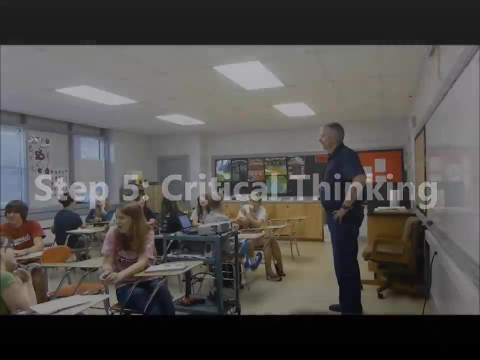 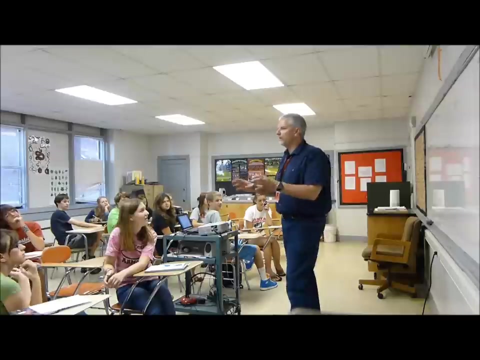 Whey, No, whey, Whey, Whey, Whey, Class, class, class, class, Yes, yes, yes, yes. Now we're gonna put this to work. I want you on your own paper, I want you to take three minutes. 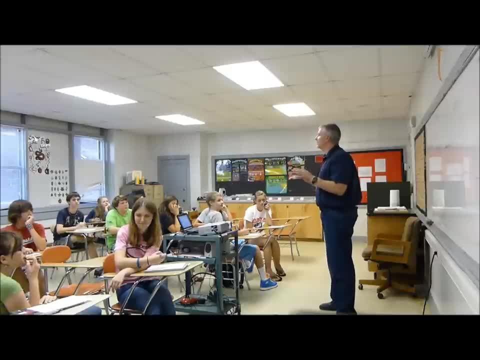 and I want you to first, without a partner. I want you to think about what you think a good definition for a chemical is, but you can't use the one I've given. you need to come up with one on your own. 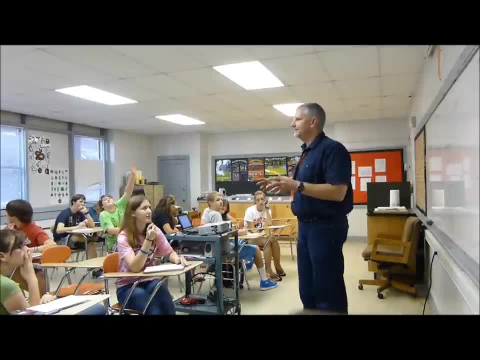 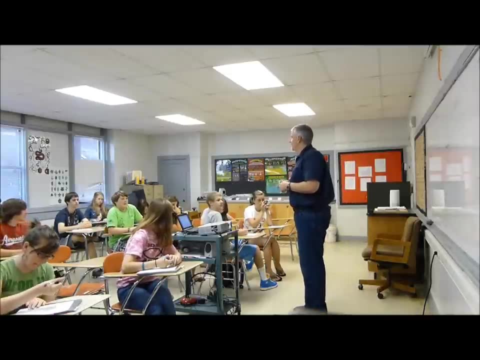 And then I want you to have your peer review, your definition, and tell them if they see any holes or what you can do to make it better. all right, Here You said a chemical one that you found right. Yeah, the one that you came up with for a chemical.